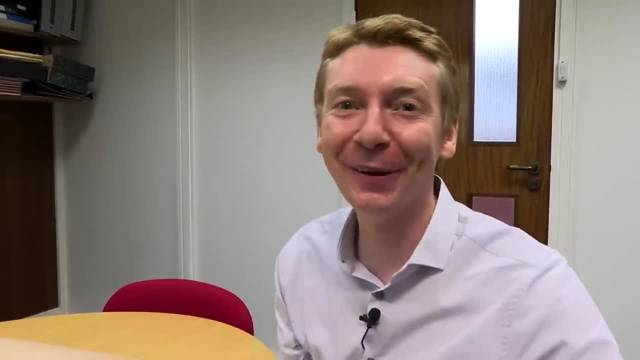 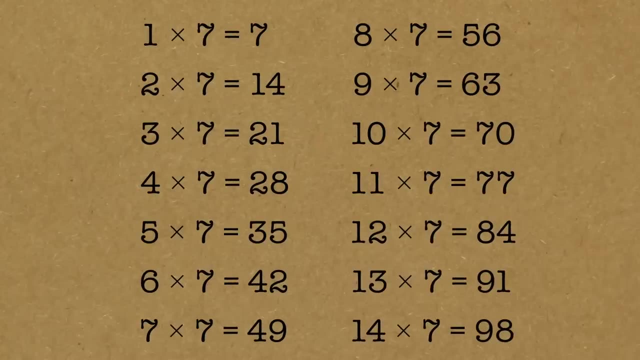 Oh, so I wanted to show you one weird trick. To work out if something's divisible by seven, you do need to know your seven times. table a little bit up to like, say, a hundred, But then if you have a larger number, this is a useful trick. So we'll pick a number. 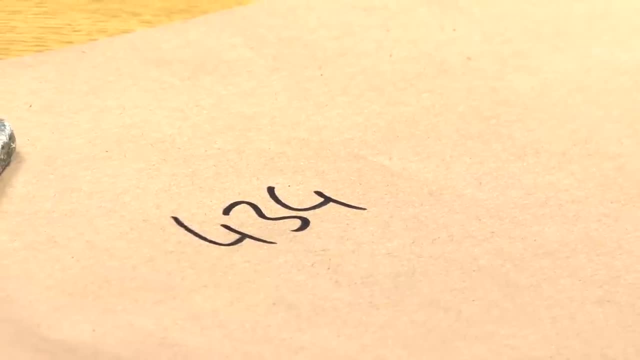 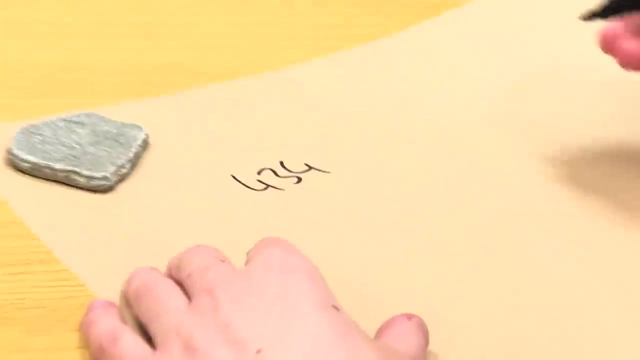 Four hundred and thirty-four. Is it divisible by seven? I don't know, just looking at it I can't tell. so this is my one weird trick: you split it up into two parts. I'm going to remove the last digit and we've got the rest. of it is 43 and the last digit as 4, and the trick. 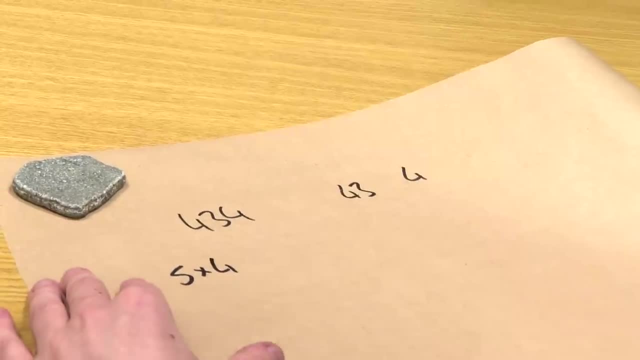 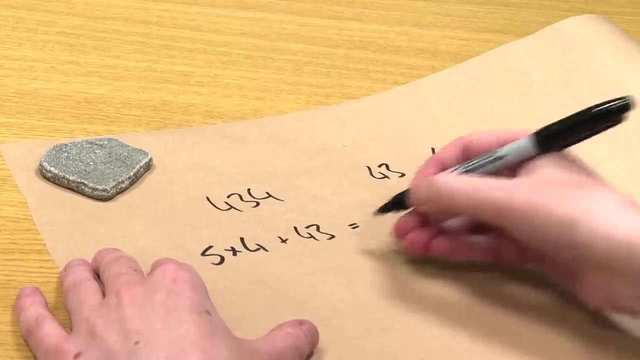 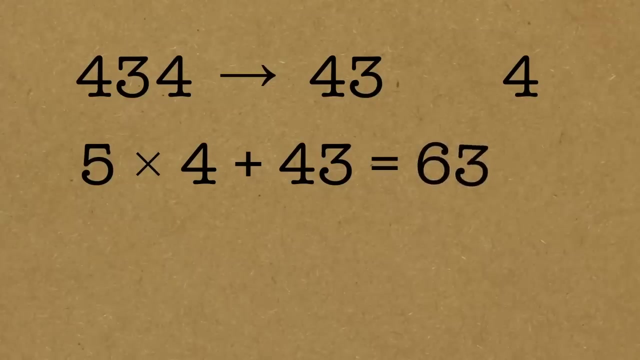 Is this 5? Times the last digit. so it's gonna be 5 times 4, plus the rest 43.. That's the little calculation I'm going to do. What have I got? I've got 20 plus 43. It's equal to 63 if that answer is divisible by seven. 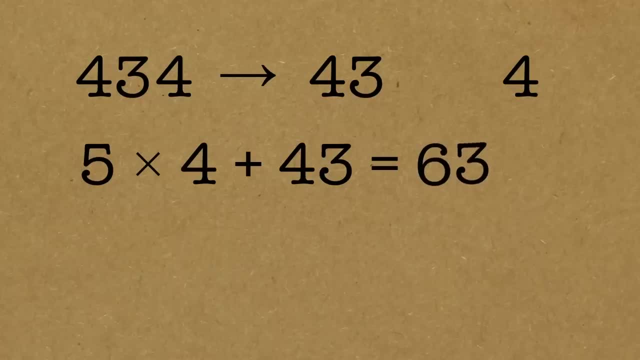 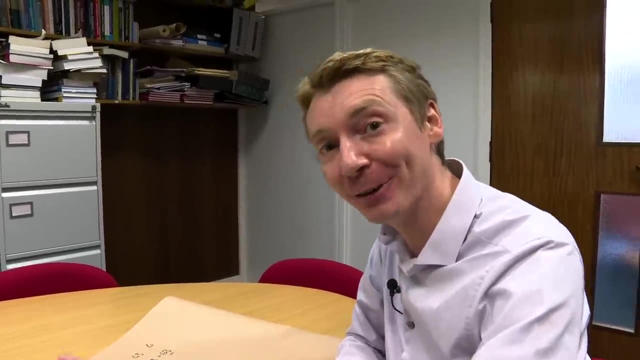 Your number was divisible by seven, and it is. that is what nine times seven. So I now know 434 is Divisible by seven. That's the little trick. It works the other way as well. if that had failed the test, if it was not a multiple of seven. 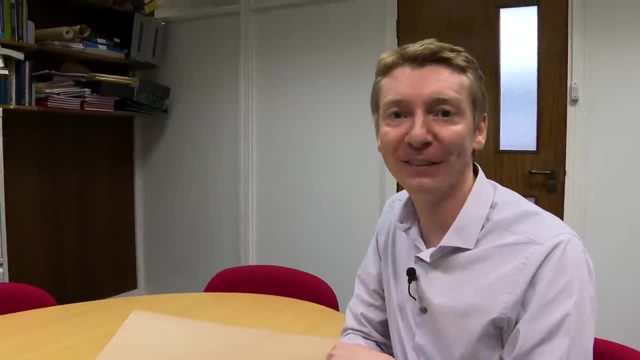 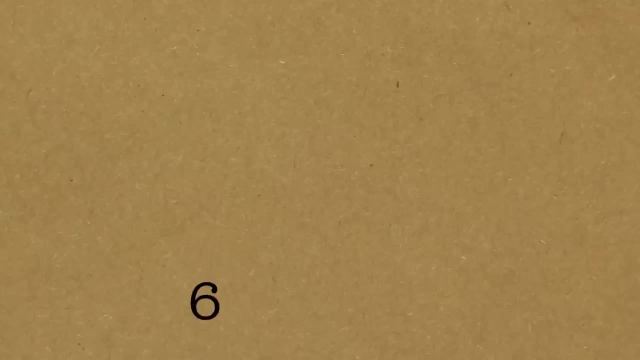 Then the original number is not a multiple of seven either, and you can even do this Repeatedly. if you got a really big number, You can actually do this a couple of times. Let's say you got a bigger number- 6468. is that divisible by seven? I don't know, I'm gonna use my trick. 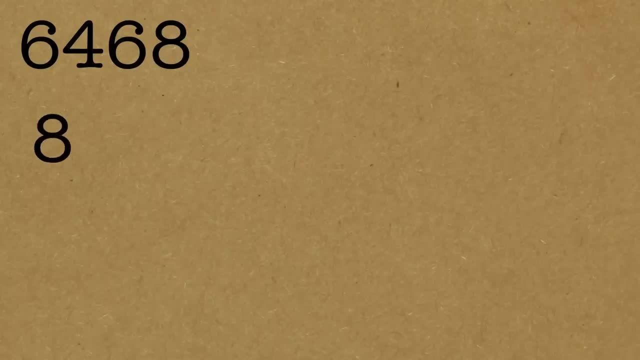 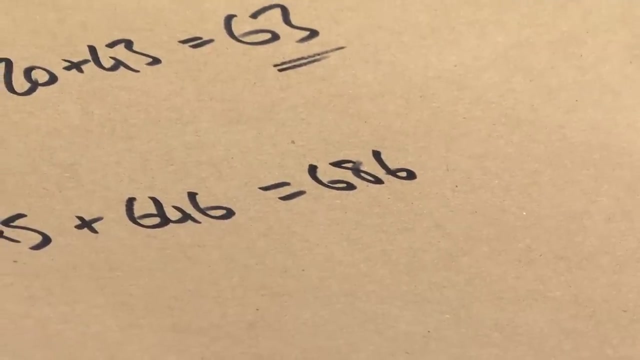 So what I can do is I take the last digit, 8, go, multiply that by 5 and I add on the rest 646. what I got here: 40 plus 646, 686. I still don't know if that's divisible by 7, But I can repeat the process. 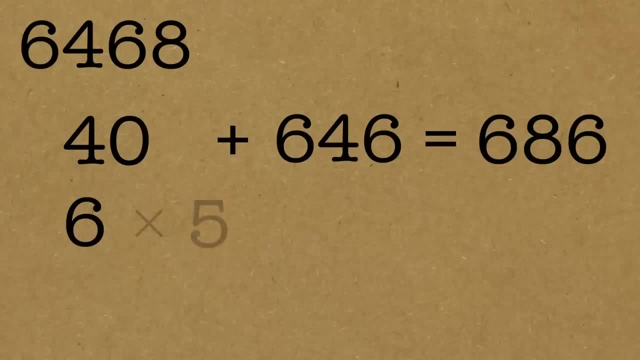 So I'll just go again. take the last digit- It's a 6 times 5, and add the rest, the 68, what I got 30 plus 68. It's 98. do you know what I could stop there? I know 98 is divisible by 7, but just for fun. 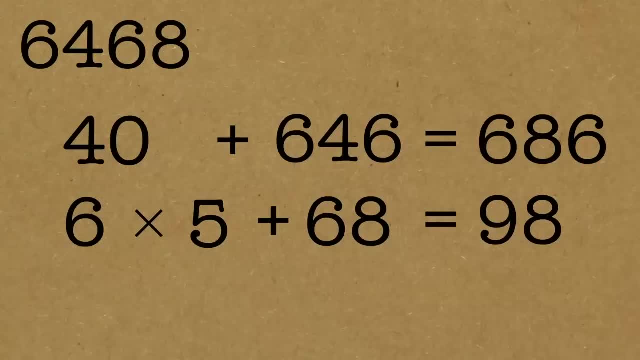 Let's take it one extra step further. Maybe you don't know: 98 is divisible by 7. last digit is 8 times 5, plus the rest, Which would just be a 9, and that would be 40 plus 9 is 49.. Yeah, I'm confident That's divisible by 7. 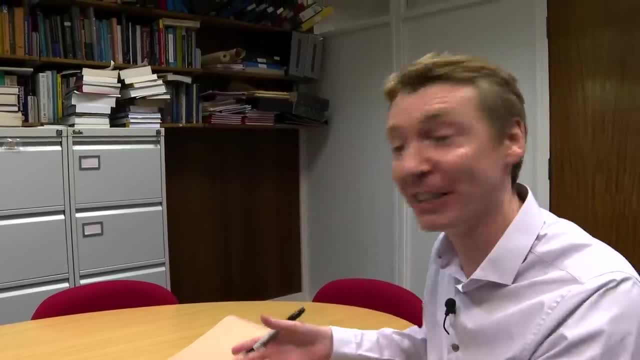 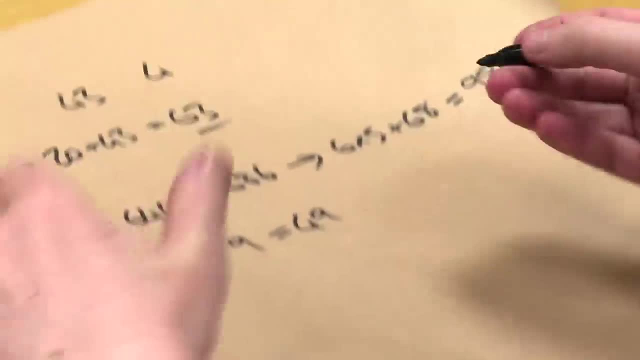 It's 7 squared and therefore my original number, which was the big number of the six thousand four hundred and sixty-eight, It's a multiple of 7.. What do you do if you do the process to 49?? Okay, let's find out. I don't know, I haven't done it. Let's find out. 49. 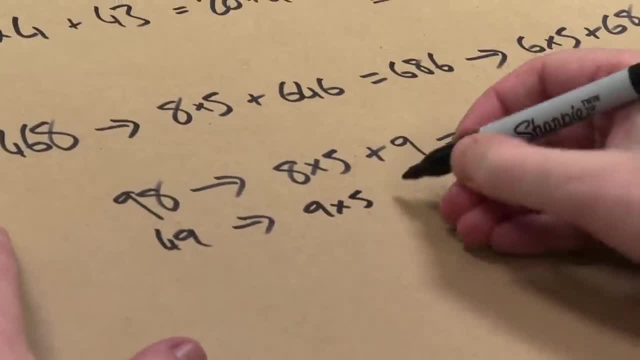 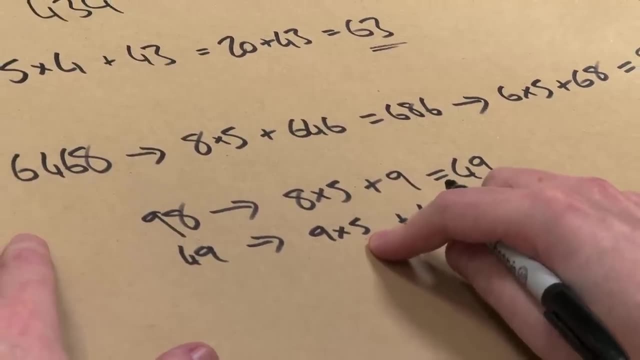 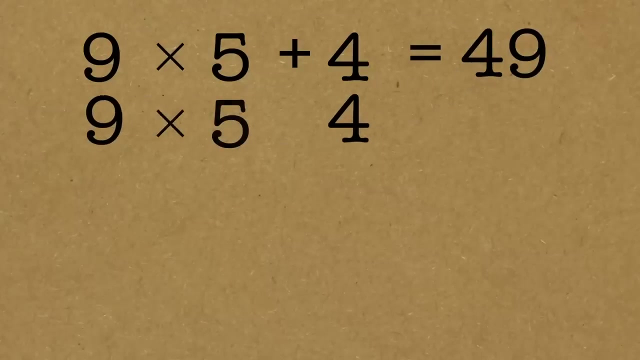 Okay, last digit is a 9 times 5 plus the rest of it, Which is just the 4, and now what we're gonna get here, 9 times 5, is 45. tell me if I'm wrong. Yeah, I got that Plus 4.. Oh, it's 49.. All right, Oh dear, We've got ourselves into a loop. 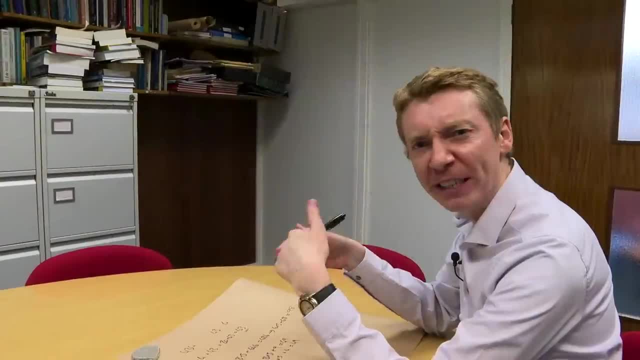 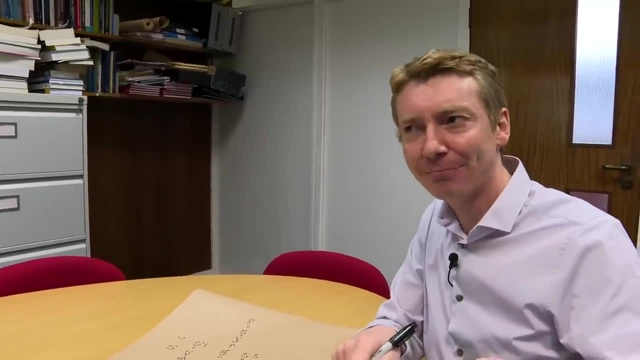 These numbers can get larger because I'm adding. With this test, I'm adding a number on, so they kind of get big, and there is an alternative version we could do which Might be more useful because the numbers get smaller. instead, I do split it up again. 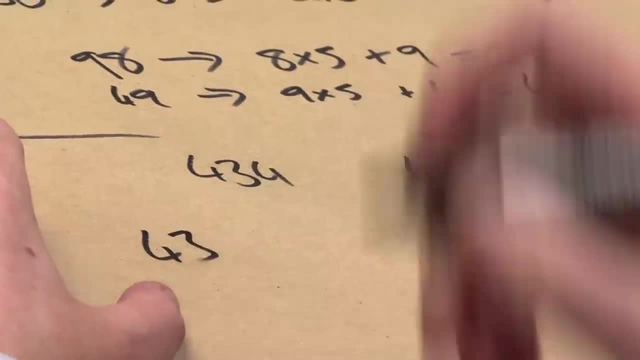 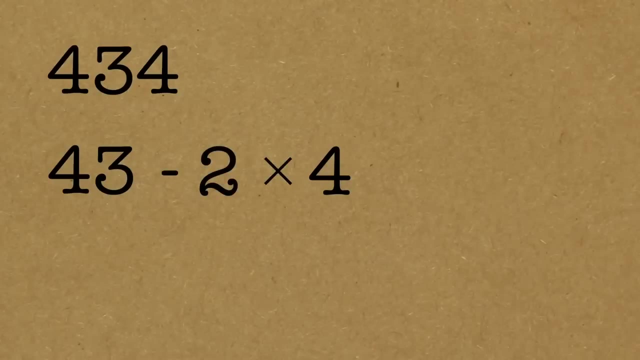 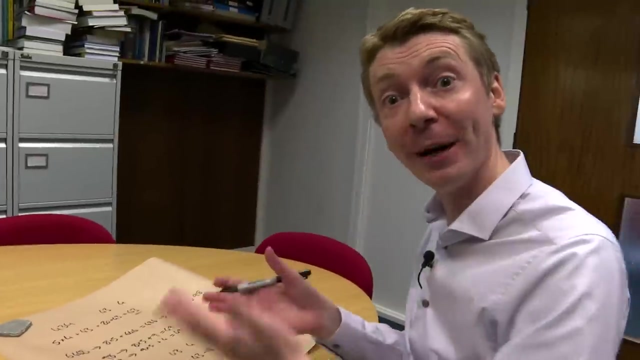 There's the 43 and 4. I take the rest as I was calling it, the 43. I subtract 2 times the last digit This time, so this time it would be 43 minus 4, 3 minus 8, which would be 35. is that divisible by 7? yes, it is. therefore my number was: 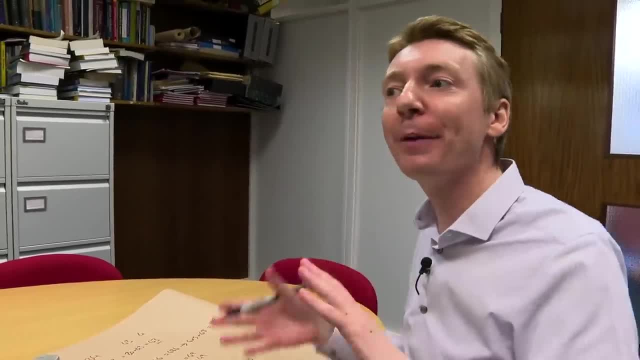 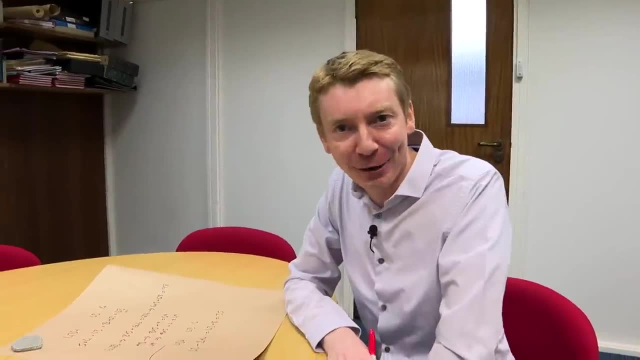 So that's a subtracting version of it, which might be more useful in some situations, may be less useful in other situations. Do you want to hear why it's true? You might want to try and work out why it's true actually, and but I am going to show you. 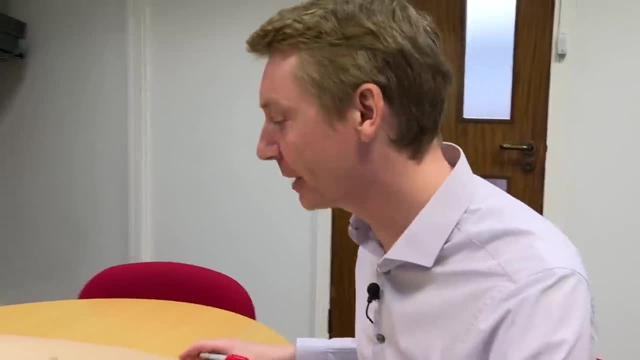 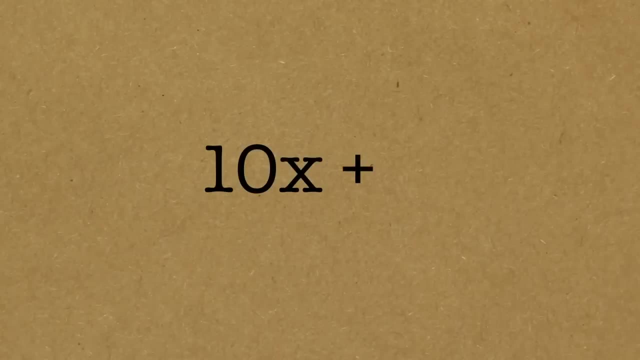 So if you want to work it out, make sure you do that. I'm gonna share how it works. Why is that true? So if I write a number, I could write a number Like this: as 10x plus y, y is the last digit and this 10x is the rest, or the X. 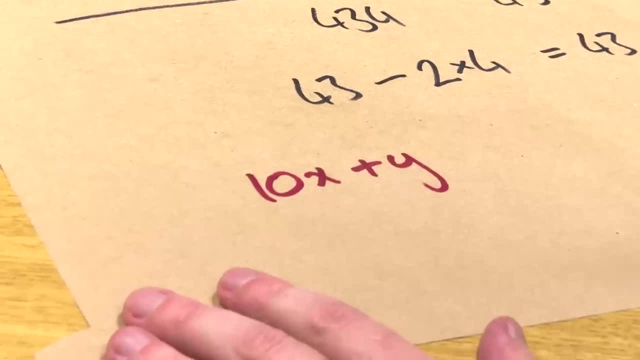 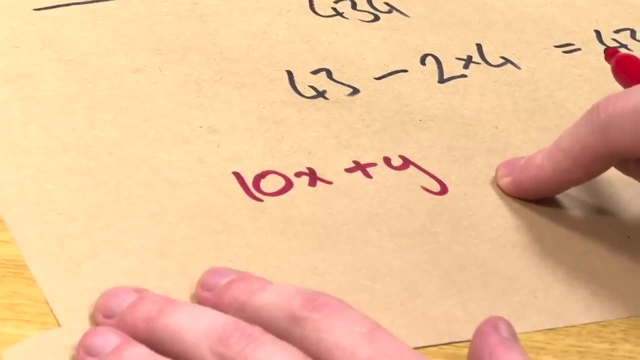 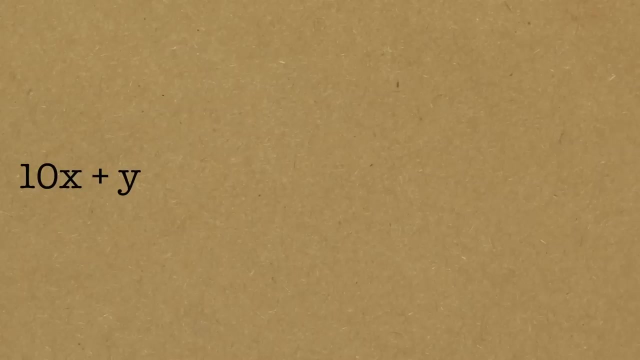 It's what I was calling the rest, That's just a different way of writing down a number. So I want to know if this is divisible by 7. I hope you would agree that if, if this is divisible by 7, 5 times, the number is divisible by 7 as well. I think that's true, isn't it? Yeah, so let's multiply this by 5. 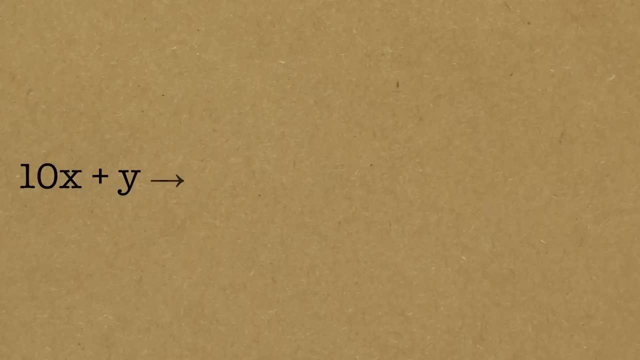 So I'm going to multiply this by 5. so what am I going to get? 50 X plus 5y. so I might want to know: is that divisible by 7? I'm going to split this up in a different way. I'm gonna have a little bracket here. I'm gonna have X plus 5y in a bracket and what's left over? 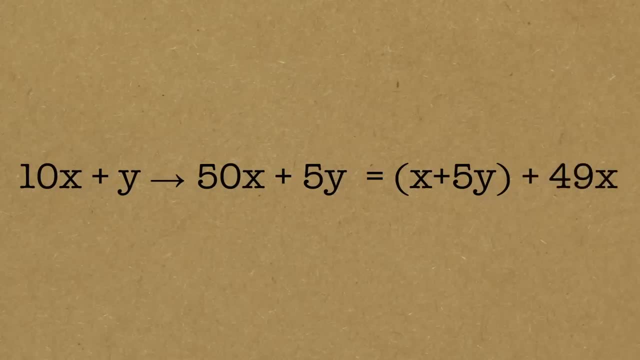 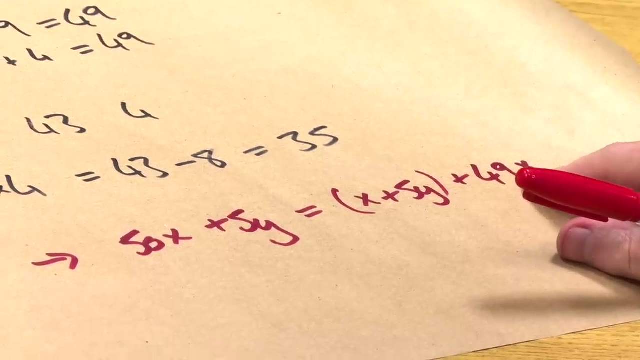 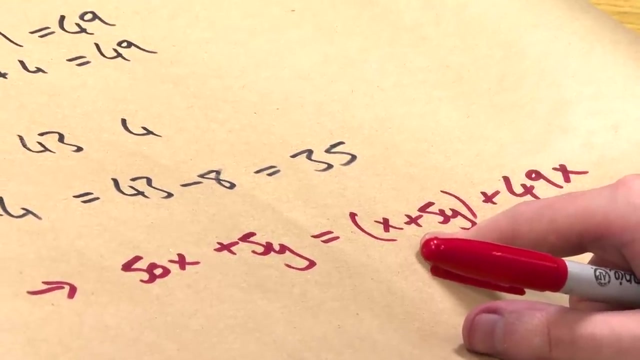 I guess it's all the X's. I haven't used this 49 X left over, So I want to know: is this divisible by 7? 49 X's definitely. I know that's definitely divisible by 7. So really the only thing that I need to ask is if that bracket is divisible by 7. 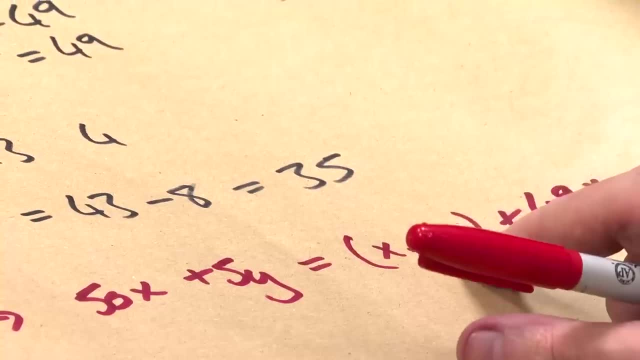 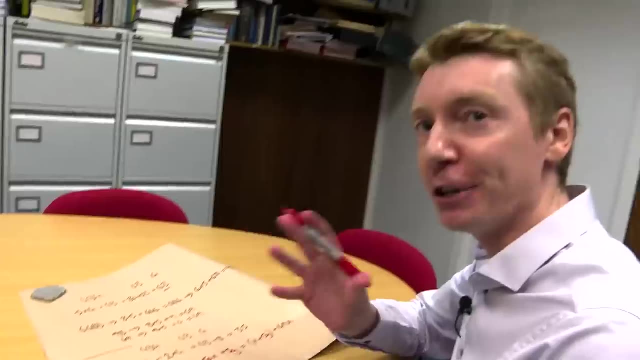 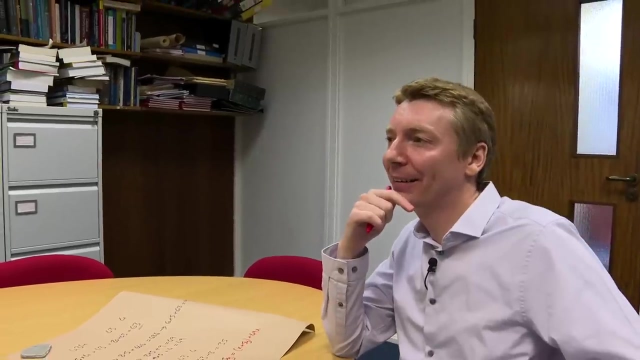 but that Bracket is my test. This is my 5 times the last digit plus the rest. So if that bracket Passes the test, if it's divisible by 7, the original number was divisible by 7, And if it's not, then the original number wasn't either. Is it ever important to know if a number is divisible by 7?? 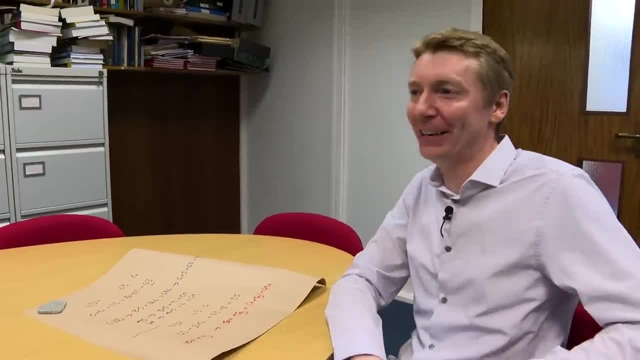 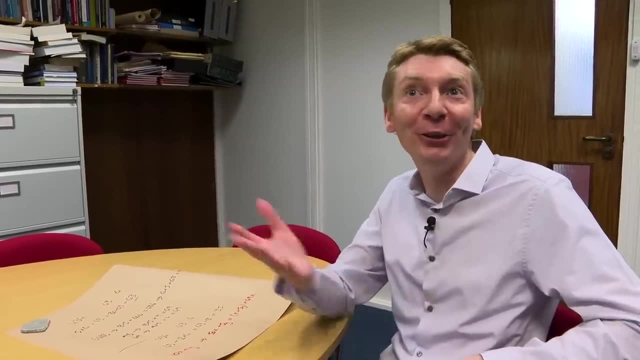 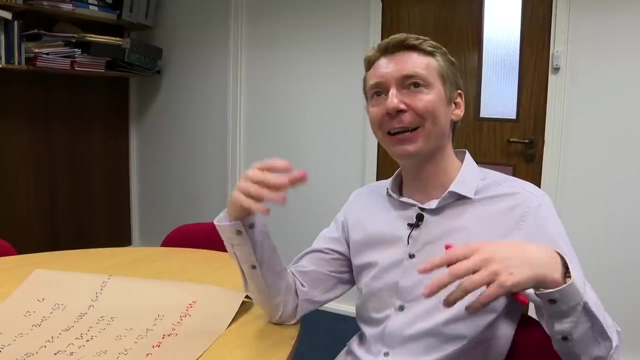 I'm sure I can think of situations where you would need to find if something is divisible by 7. I mean it's more useful to know when things are divisible by 4 or 2 or 6 is kind of useful and 7 is less useful if- unless you're going to like a restaurant and you've got 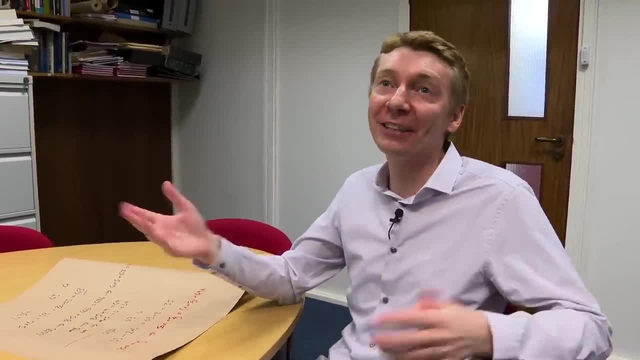 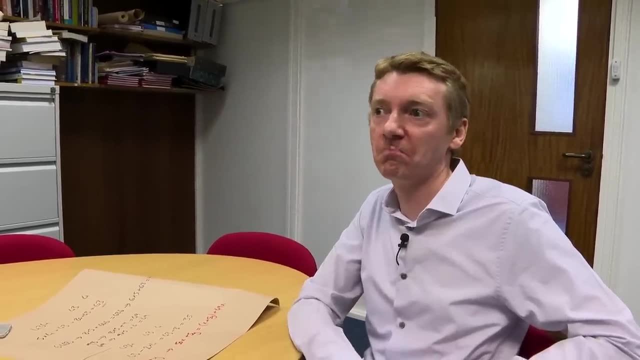 7 people and you want to split the bill. you know that kind of thing. So I can't imagine Rugby, maybe converted tries in rugby, or a touchdown with a field goal with a conversion, a Touchdown with a conversion, seven points. Yeah, look at my face. Look how blank my face is now. 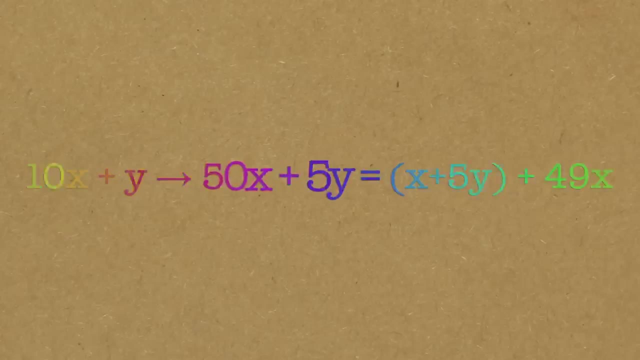 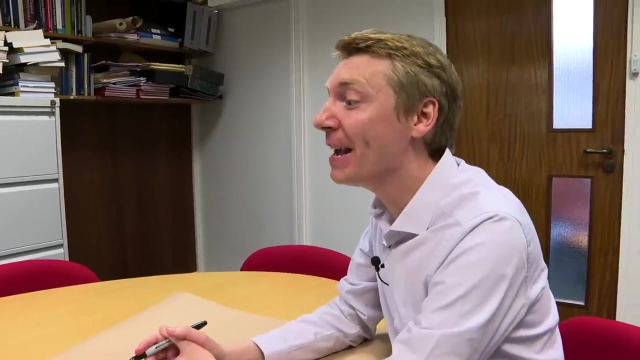 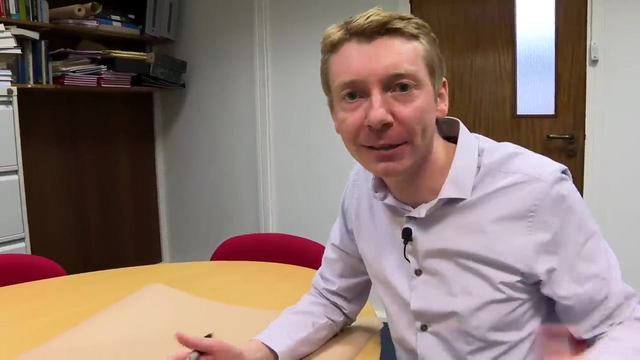 I have no idea what you're talking about, But maths is good, isn't it? Now that we've seen a test for the divisibility of 7, Maybe it's nice to do a recap of some of the tests for smaller numbers And now you might be useful. keep them in your pocket and then you'll know them. 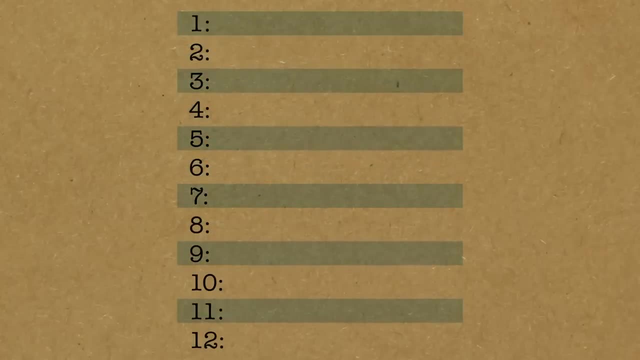 right how to tell if your number is Divisible 7. we know, we've now got a test for this and it was the 5 times last digit plus rest. Awesome, tick 1.. Well, everything's divisible by 1.. Okay, I'll just write that in there. 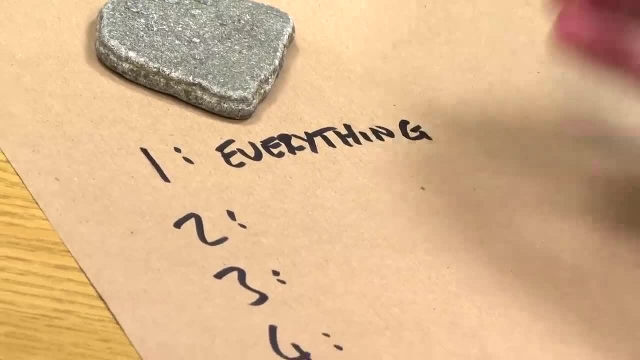 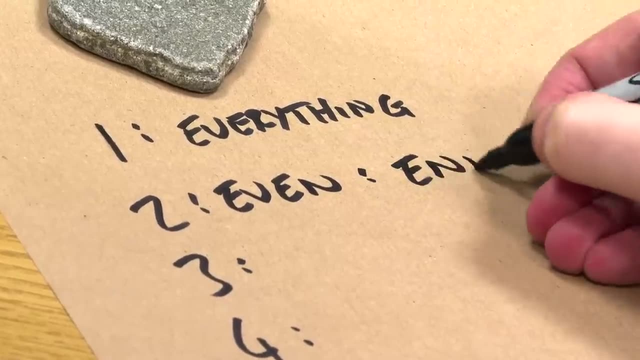 Everything, let's do the easy ones next. and divisible by 2, Even, right, even numbers. but another way of saying even is the end with a 0, a 2, a 4 or an 8, and Then you know it's 6.. Oh, 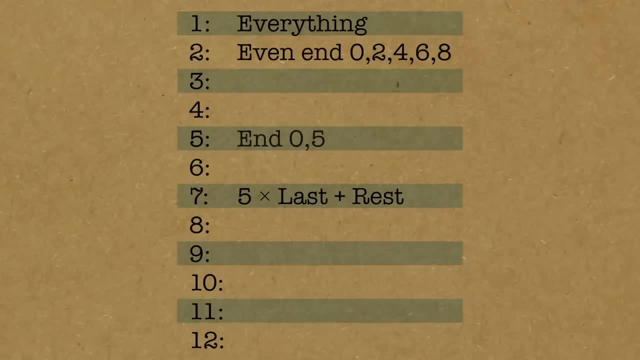 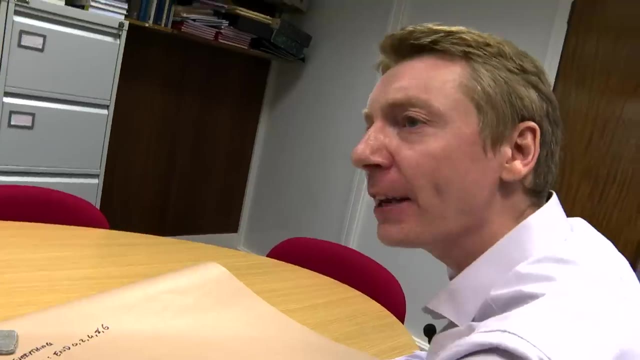 And 5 is an easy one as well, isn't? it ends with a 0, or 5?? Yeah. and 10 is an easy one. ends with a 0. cool, Those are the easy ones. the next easiest test: I think it's divisible by 9. 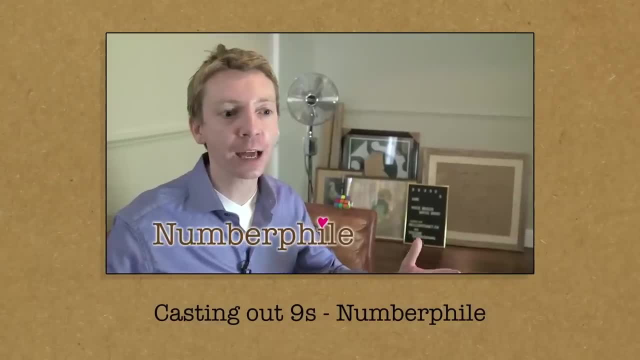 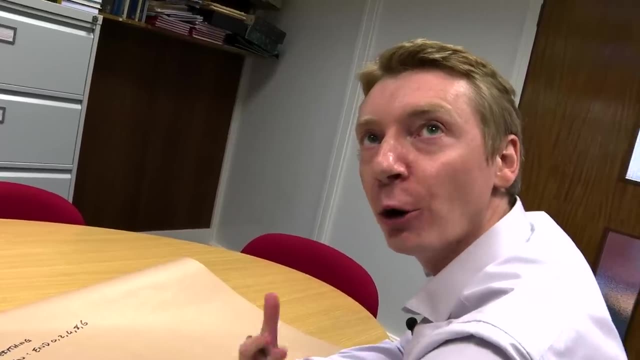 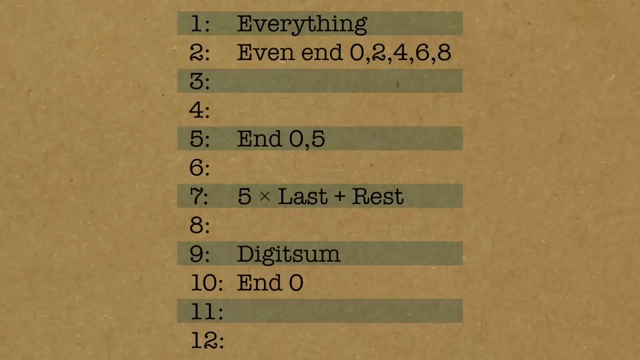 I've actually done a video about divisible by 9, a trick that can check your arithmetic, But I think this is something that everyone should know before we called it casting out nines or the rule of 9, and the test For this is something called the digit sum. We add up all the digits and if the digit sum is divisible by 9, 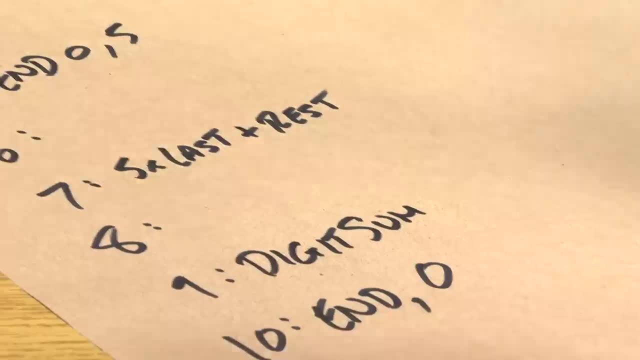 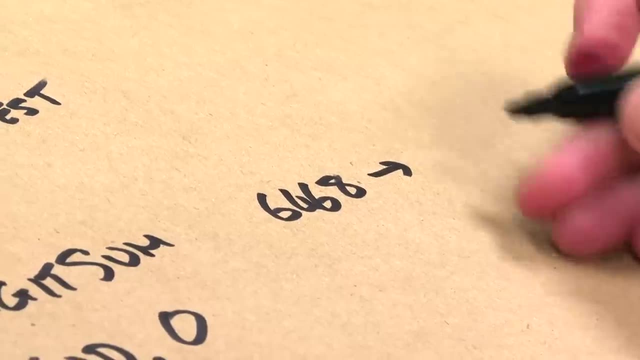 Tick. the original number was- let's just do an example, I'll steal the example I did before- right, 6468. So the digit sum would be adding up to The digits 6 plus 4 plus 6 plus 8. what if I got there? 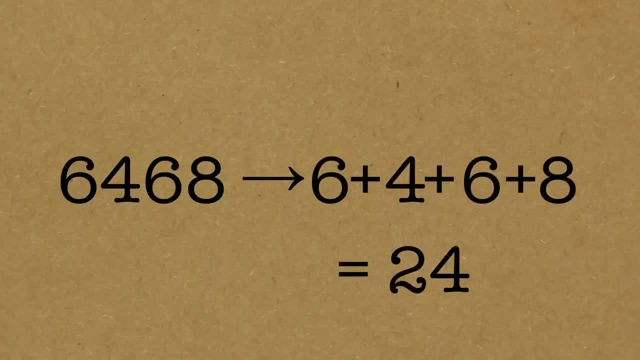 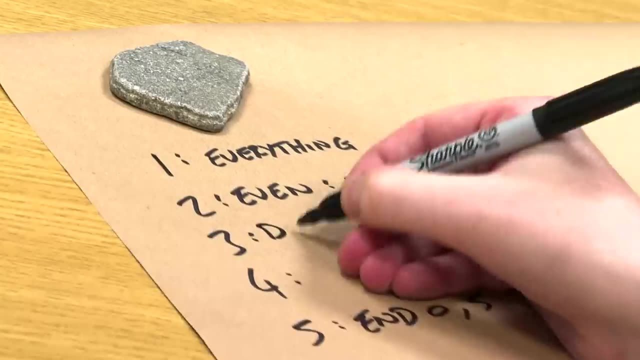 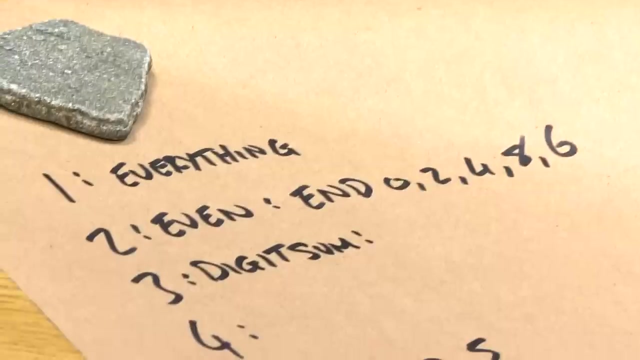 10, 16, 24, which I guess means it's not divisible by 9. that failed the divisibility test, But it does pass the test for 3. the test for 3 is the digit sum. again this time, if the digit sum is Divisible by 3, the original number was divisible by 3, 11.. Shall we have a look at the test for 11?? 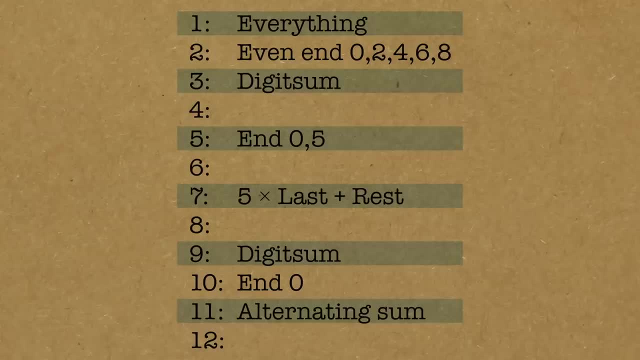 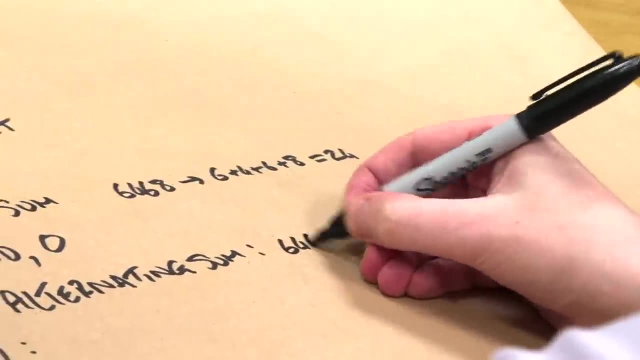 That's the alternating sum. It's the same idea really. you alternate the plus and minuses. Let's do that example to show you what I mean. So I had this number again: the. the 6468 start with the 6. You subtract the 4, you add the 6. you subtract an 8. 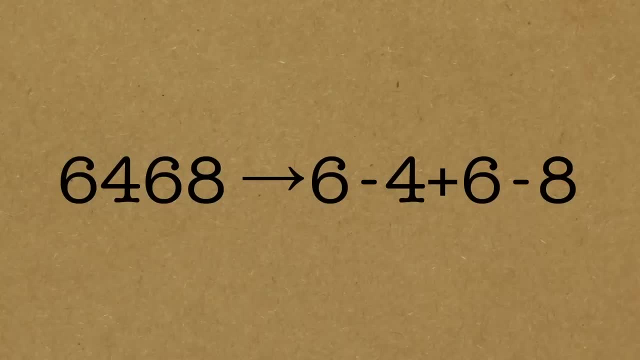 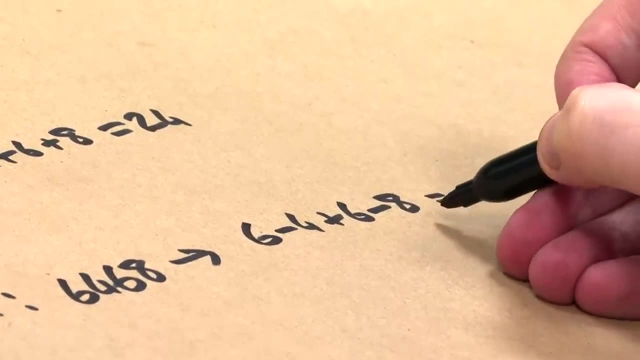 So you keep a plus and minus in the digits like that. If that's 0 or multiple of 11, it passes the test. What if I got here? It's a 2 and 8 minus an 8 is a zero. That's ok. 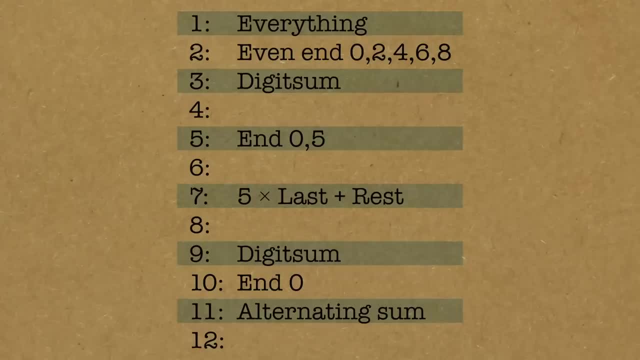 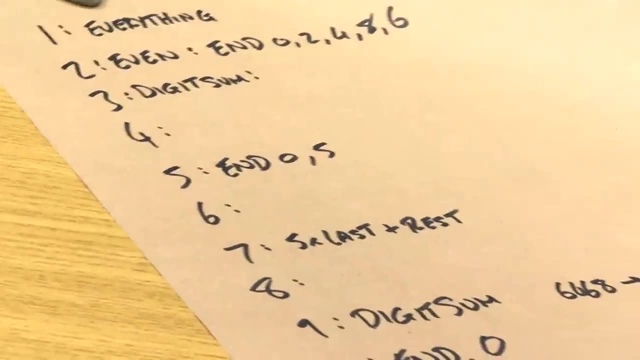 so if it's a 0, it passes the test. that means it's a multiple of 11.. My number was a multiple of 11.. All right, so what have we got left? The next easiest one is 6.. How do we know if it's divisible by 6? Well, all you do is you apply two. 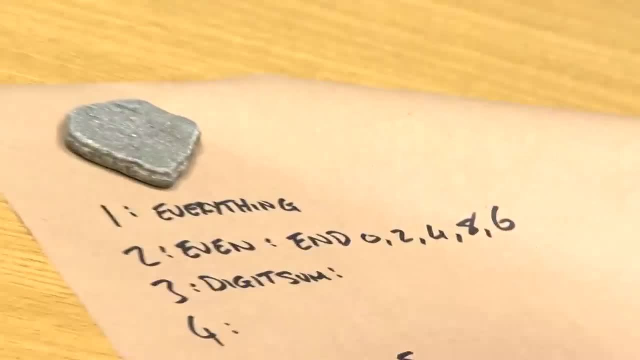 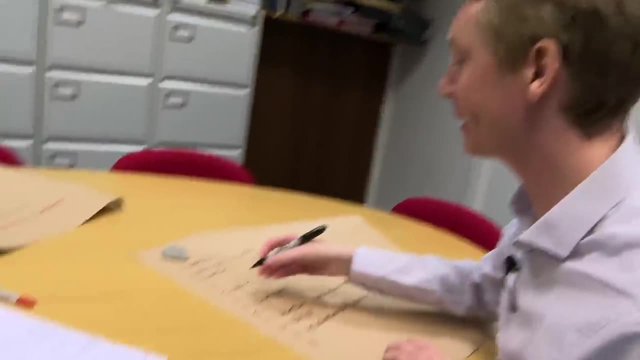 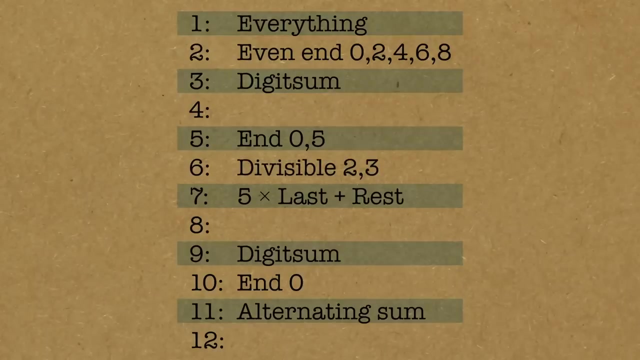 tests. Does it pass divisibility by 2 and divisibility by 3?? If it does, then it's divisible by 6.. So you have to pass two tests: divisibility by 2 and 3.. What about my example? I've been using 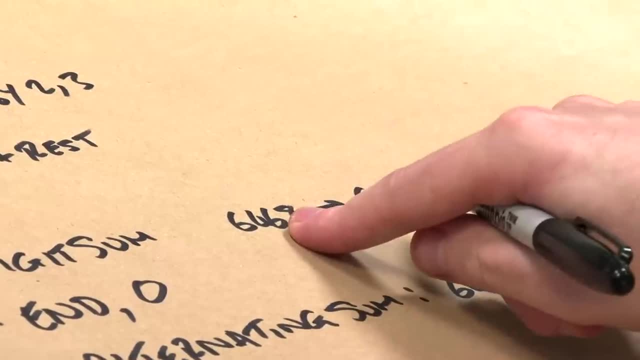 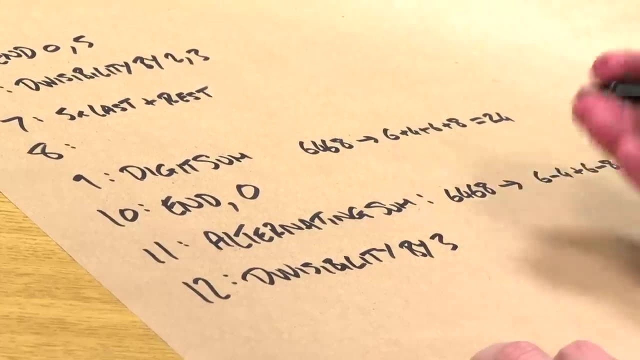 the 6468?? Yeah, I mean it passed the 3 test and it passes the even test, so it's divisible by 6.. You do the 12 the same way, so it just needs to pass divisibility by 3 and 4.. Oh, I haven't done. 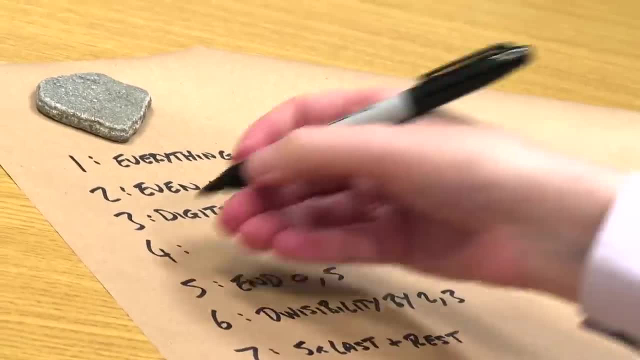 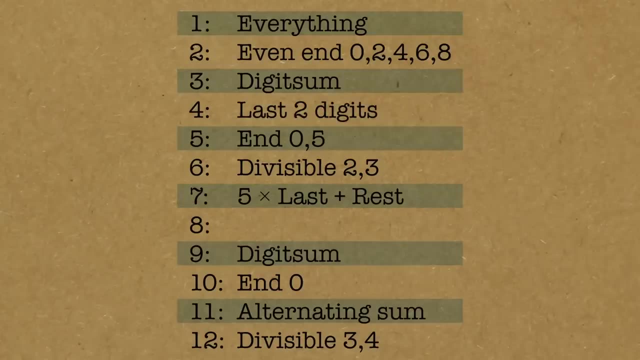 4, so I should mention it: 4,. what is the divisibility by 4 test? You look at the last two digits. Let's use my example here. I just care about the 68. I really don't care how. 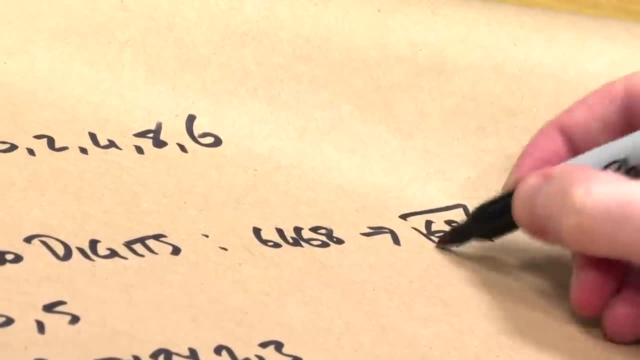 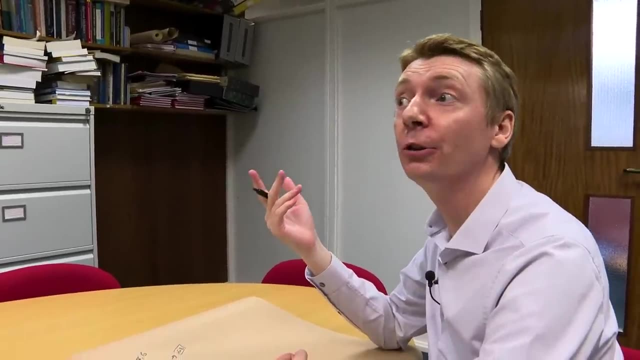 big this number is either It's just the 68 I care about. And then, is that divisible by 4?? You might think, but is that hard working out? if that's divisible by 4? I like to do. can I divide by 2? 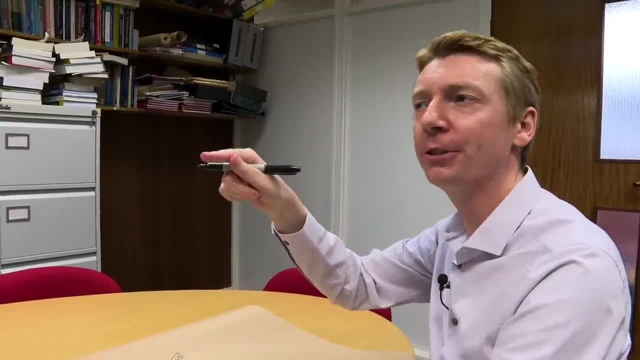 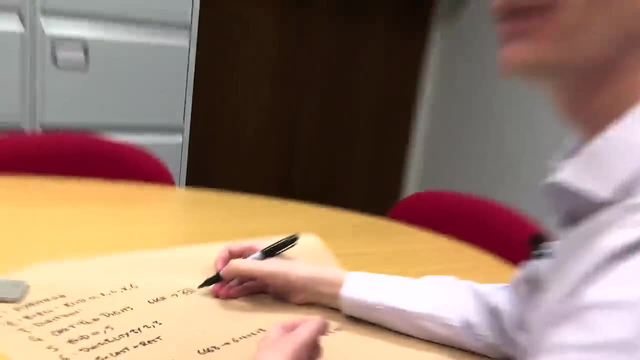 twice, Is it doubly even? So is it. can I divide by 2, and is that even I can divide by 2 again? So if I did that, 68, is it doubly even? It'd be 34,. and then, yeah, that's even, which would be a 17 if I halved it again. That passes. 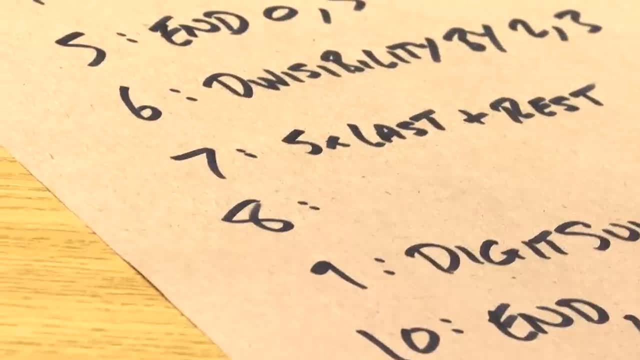 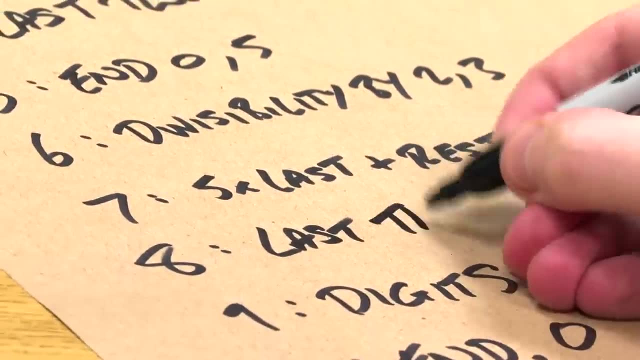 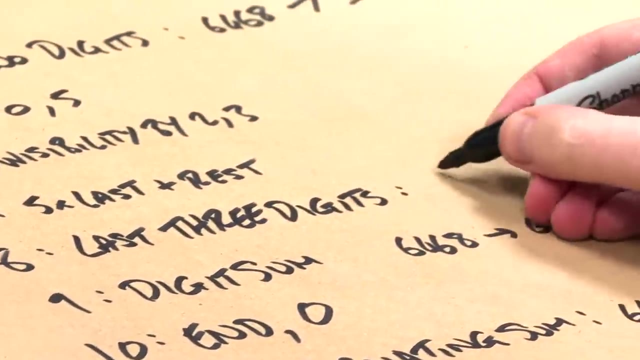 And for 8, this is the, apart from 7, I say 8 is maybe the harder one. it's the last 3 digits. Don't care how big the number is, but it's the last 3 digits And I'll do my little. example: Here's my 6468.. I only care about the end of it, the 4,. 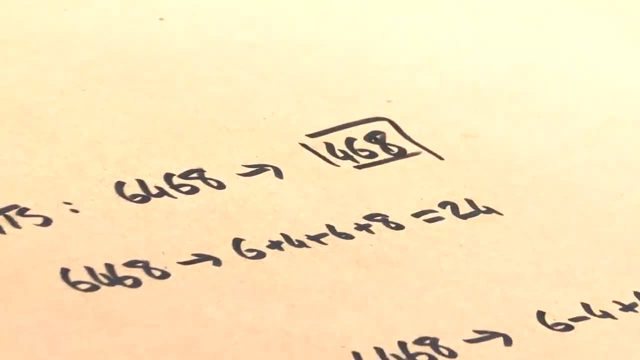 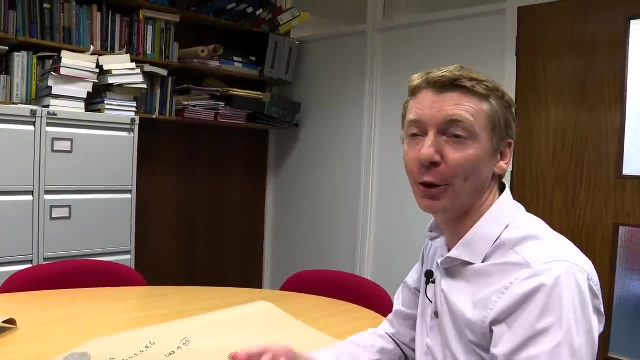 6, 8 part, There it is. Is that divisible by 8?? That's again kind of hard. Is it triply even Then? So is it even. Can I divide by 2?? Can I divide by 2?? Can I divide by 2??